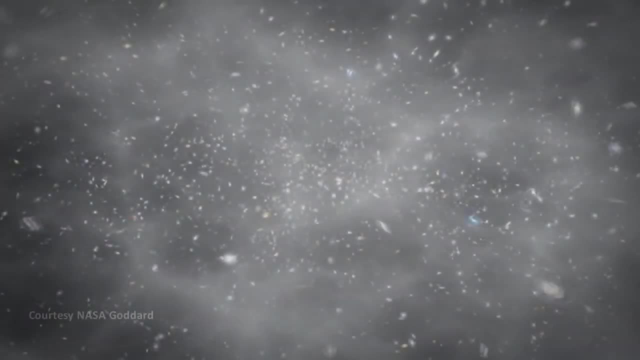 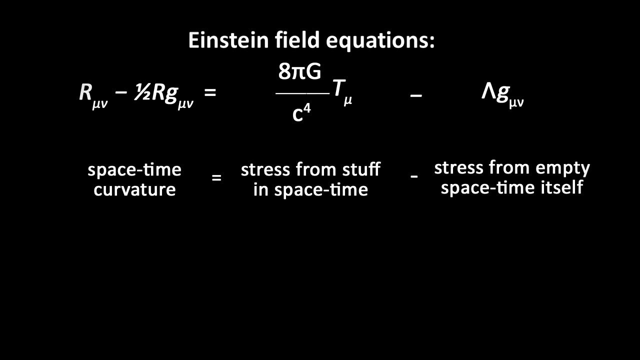 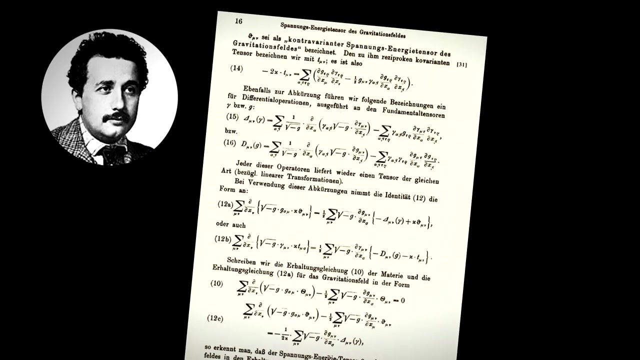 biggest pursuits in physics is the attempt to find a better theory, a quantum theory, of gravity. In order to understand quantum gravity, though, you have to first understand general relativity. However, the mathematics of general relativity is so difficult that even a genius like Einstein 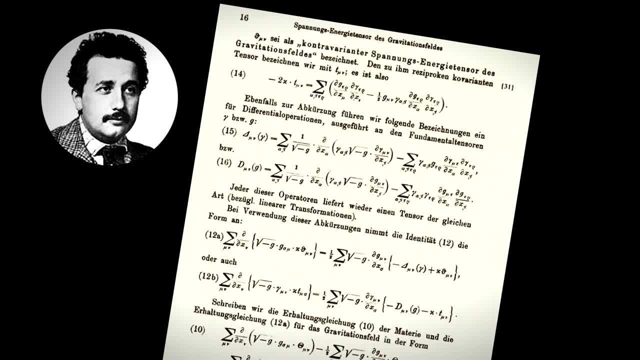 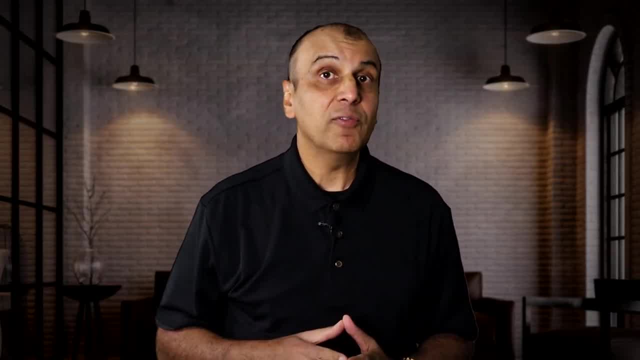 could not easily solve a puzzle of minor equations that required the use of high and low degrees. not easily derive it, And there are still papers being written today on specific solutions to these equations. I'm going to try to explain those equations to you intuitively and visually. to 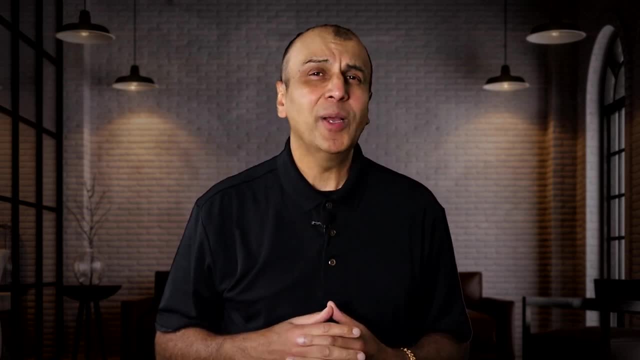 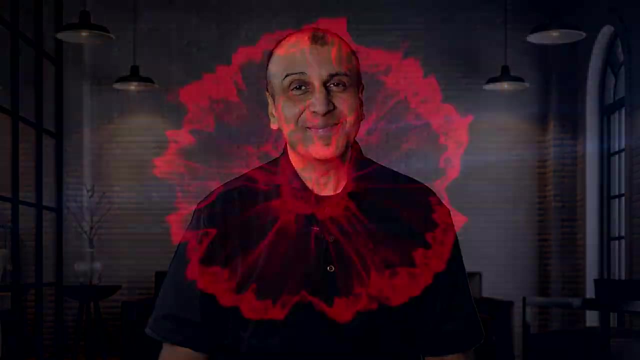 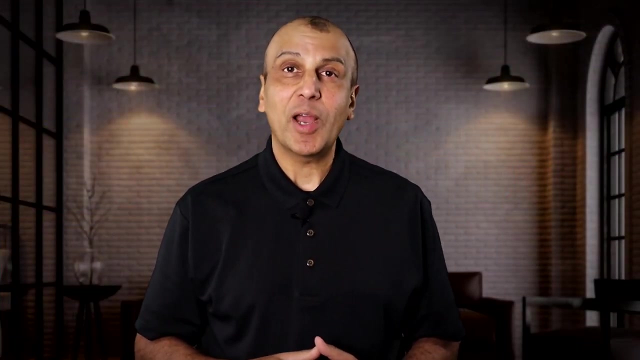 give you an idea of what the math is trying to say, And I hope that this will help you better understand quantum gravity. That explanation is coming up right now. Before I get into general relativity and quantum gravity, let me tell you part of my inspiration. 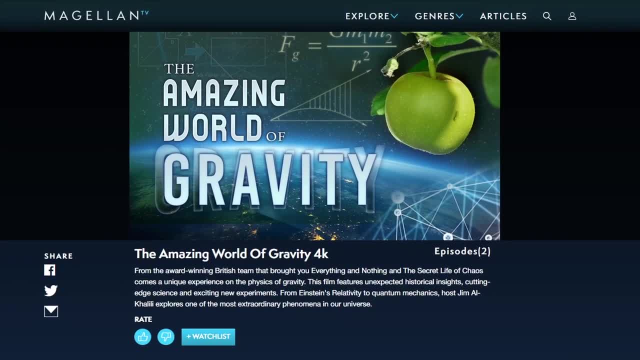 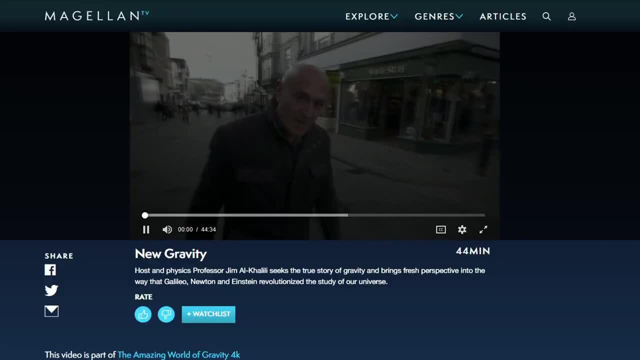 for doing this video. I watched a fascinating two-episode documentary on Magellan TV, today's sponsor, called The Amazing World of Gravity. It's not only in 4k but also hosted by one of my favorite educators, Jim Al-Khalili. Magellan is a new type of streaming documentary service, founded. 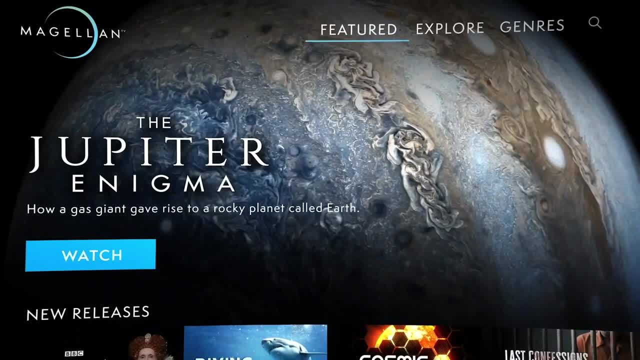 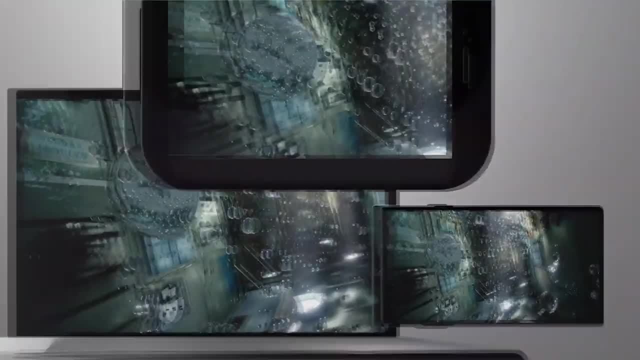 by filmmakers and producers who bring premium, in-depth documentary content. Featured subjects include history, nature and- my favorites- science and space. You can watch it on any of your devices, as well as your TV, anytime, without any ads, and they have a huge library of. 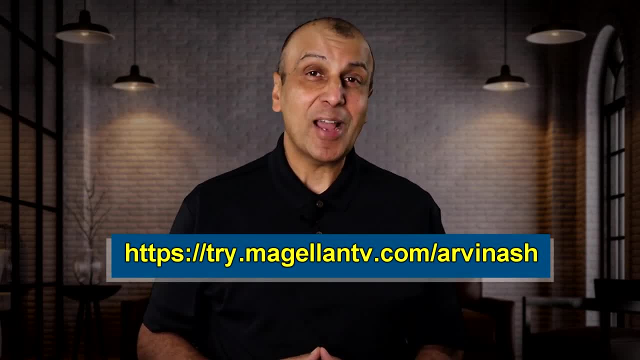 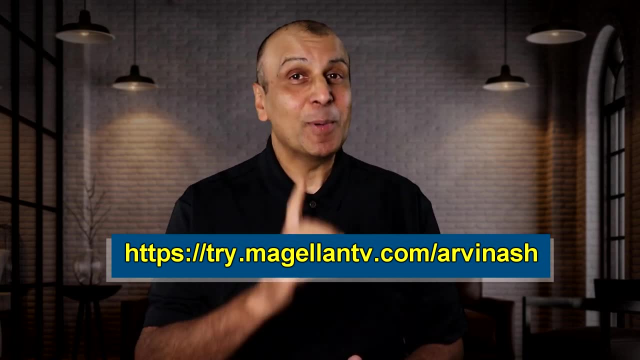 4k content. Magellan TV has a special offer right now for Arvin Ash viewers. If you use the link in the description, you will get a free one-month trial. I highly recommend Magellan TV. Be sure to use the link in the description. If we look at Newton's equation for gravitation and Einstein's, 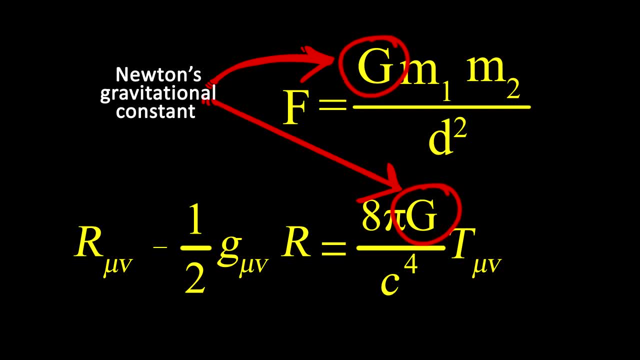 equation for general relativity, we see that the equation for gravitation is the equation for gravitation. If we look at Newton's equation for gravitation and Einstein's equation for general relativity, we see a remarkable correlation. For one thing, Newton's gravitational constant is: 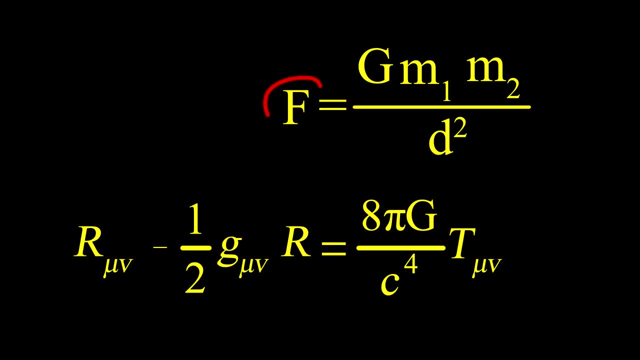 present in both equations. In Newton's equation we have a force on the left side created by a mass on the right side. In Einstein's equation, we have the analog of force, the curvature of space-time, on the left side. It has two components that describe the curvature and how distances in 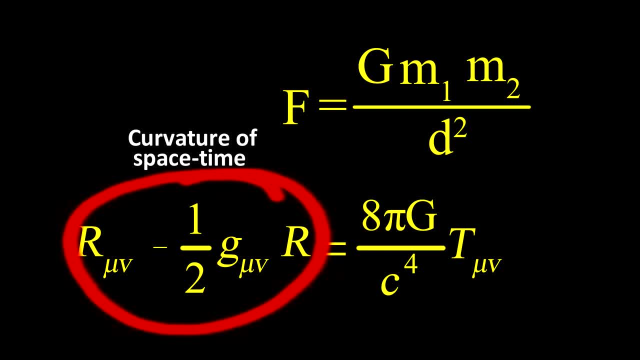 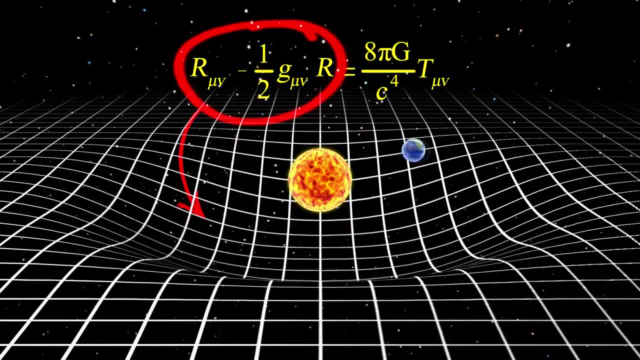 the curvature are determined. This is the analog of force described by Newton. I want to be careful here, because in general relativity gravity is not a force within the background of space time, like it is in Newton's equation, but it is a curvature of the space-time background itself. 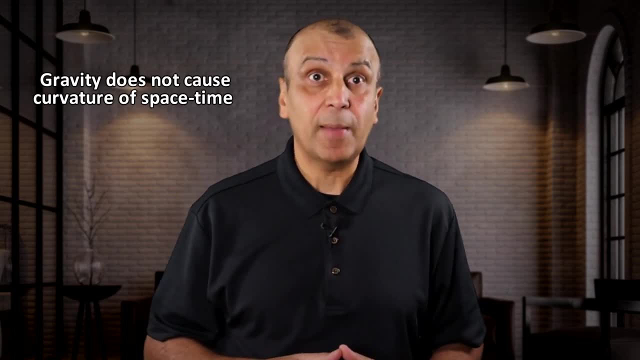 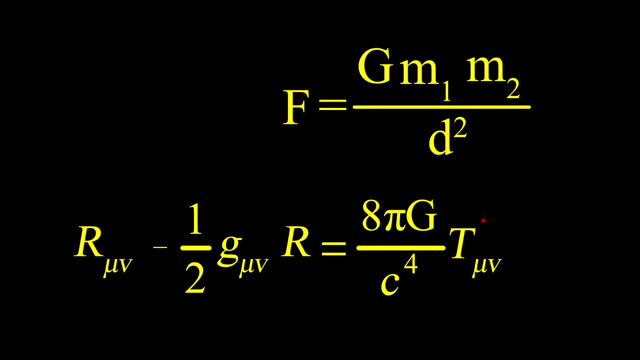 In other words, gravity does not cause the curvature of space-time, It is the curvature of space-time. The right side of the general relativity equation tells us about the mass energy content. This is represented by something called the mass energy momentum tensor. It's a 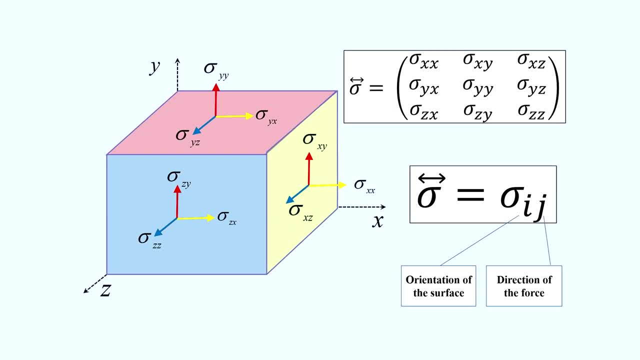 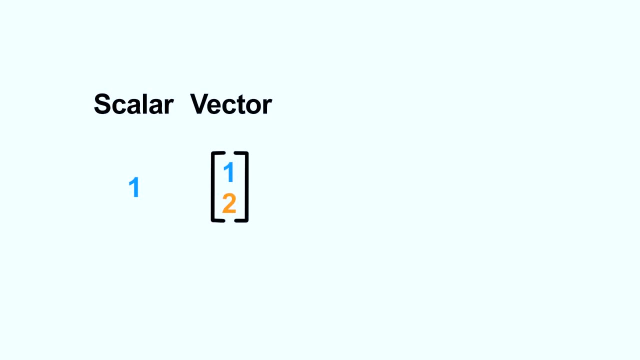 source of the curvature. In the context of these equations, think of a tensor as a multi-dimensional array of mass-energy momentum. The mass-energy momentum tensor is the mass-energy momentum mathematical components. This can be an array of vectors, scalars or other tensors, and it's. 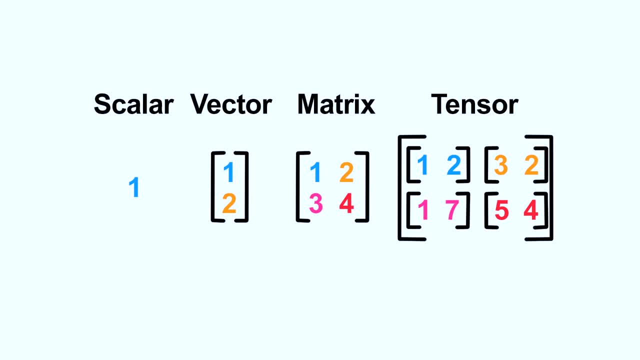 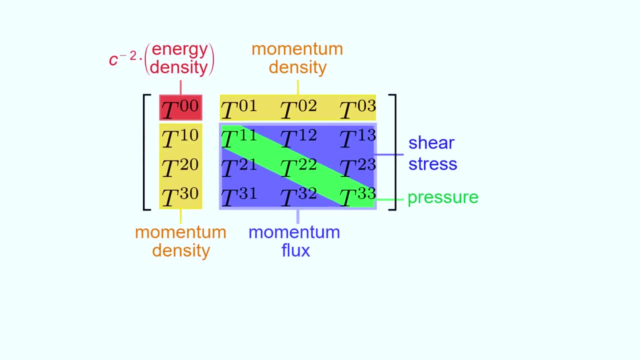 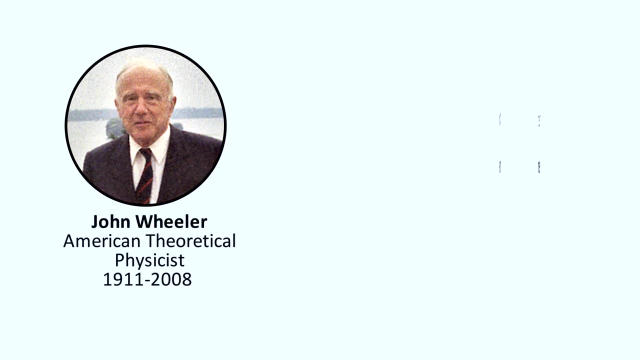 represented by an n by n matrix. A vector is a type of tensor represented by an n by 1 matrix. In general relativity the dimensions are four, so the vectors are four by one and the tensors are four by four matrices. So this equation describes what John Wheeler said. 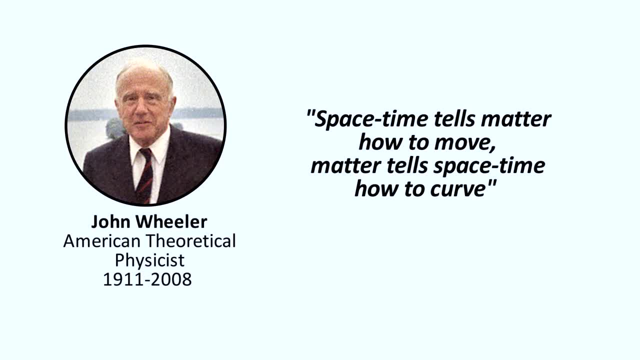 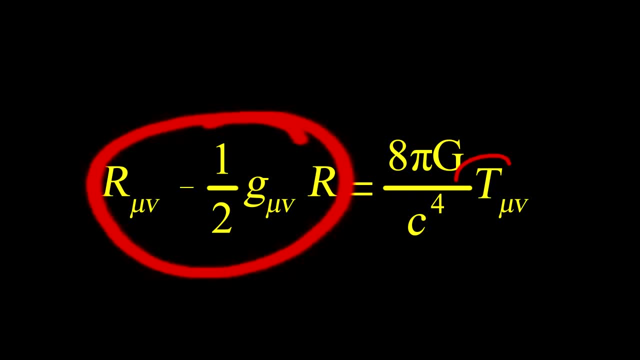 so succinctly about general relativity. Space-time tells matter how to move. matter tells space-time how to curve. The right side is the matter and energy which tells space-time on the left side how to curve, In return, the left side. 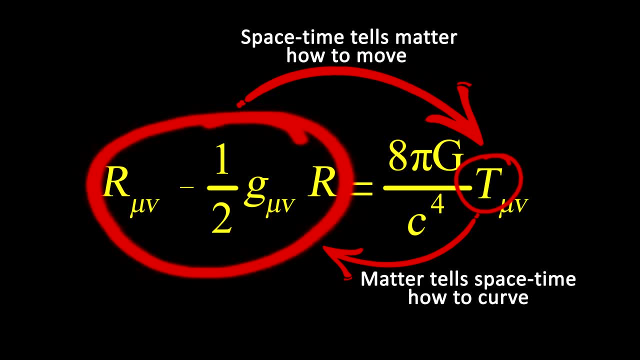 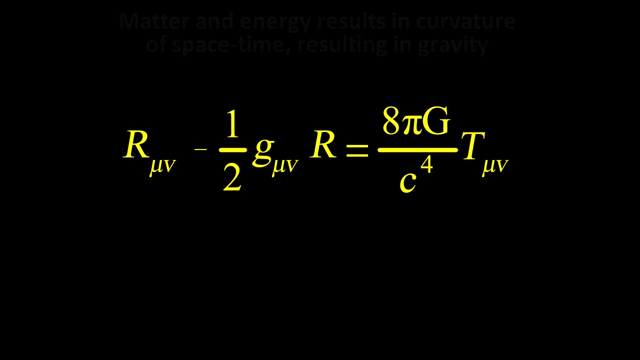 the curvature resulting in gravity tells matter on the right side how to move. Essentially, what this equation shows is that matter and energy results in a curvature of space-time which we perceive as gravity. Although this looks like one somewhat simple equation, it is actually ten equations. 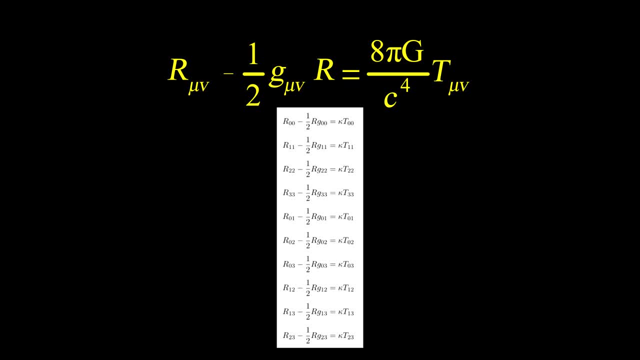 And it is very complicated mathematically. If we wrote down all the ten equations fully, it would take up more than a page of text. A simplified version is shown here. It is so complicated, in fact, that Einstein was skeptical about being able to solve them. 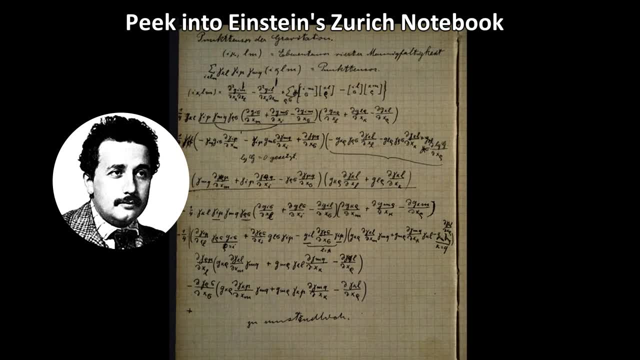 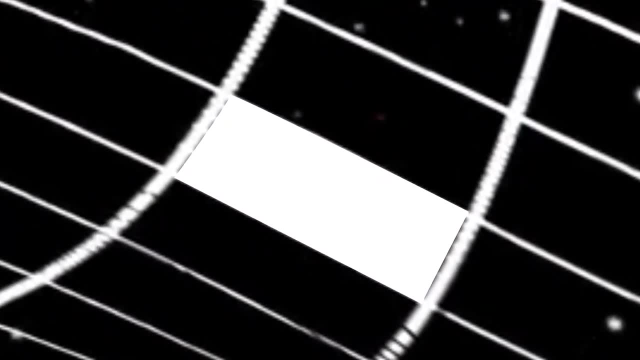 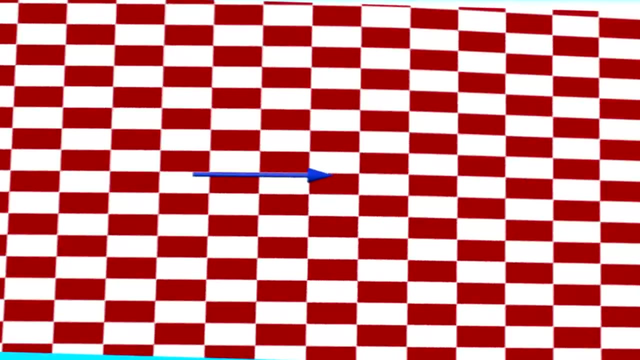 There are papers written to this day on various solutions to these equations. Let's take a closer look at what these equations are trying to say. The equations describe the curvature of space-time by treating it as being flat at infinitesimally small distances. So you can consider that general relativity behaves like. 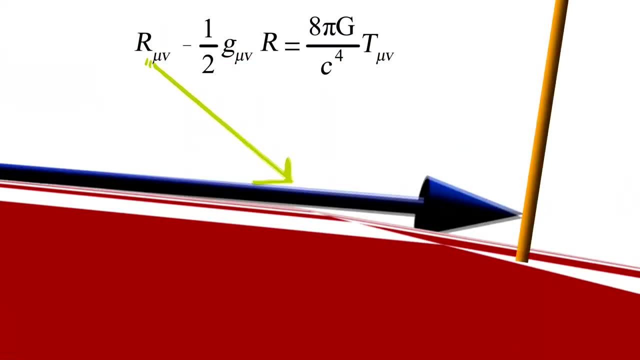 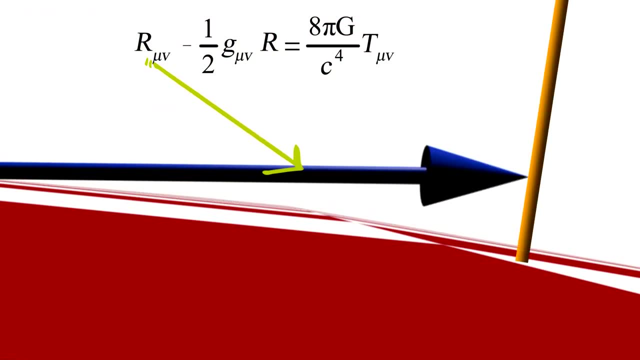 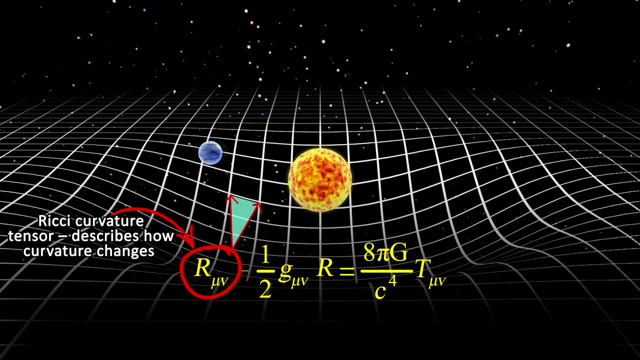 special relativity at these small distances with no bending or curvature, But overall curvature is taken into account. r mu nu is the Ricci curvature tensor. It tells us how space-time is deviating from flat. It tells you how space-time curves at a given point. 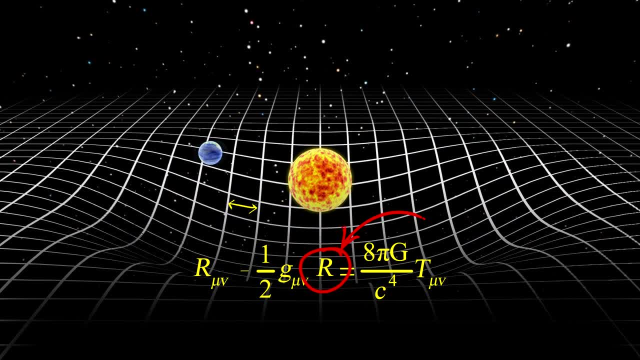 The second term on the left side is composed of: r, the scalar curvature. It tells you how much the space is changed at any given point, such that you know how to correctly measure distances. Little g, mu nu is the metric tensor. It tells you the geometry and structure of space-time. 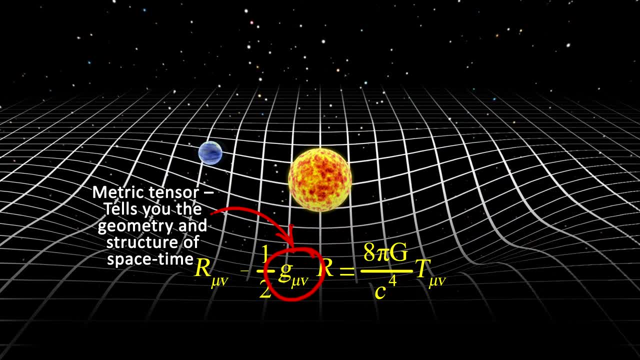 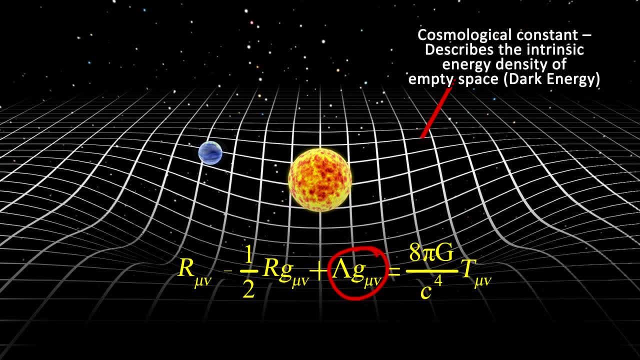 Together. this term defines how distances are calculated given a curvature at any point. Note that sometimes a third term is added: lambda times g, mu, nu. Lambda is the cosmological constant. This term describes the intrinsic energy density of the vacuum or empty space. It's the mathematical expression. 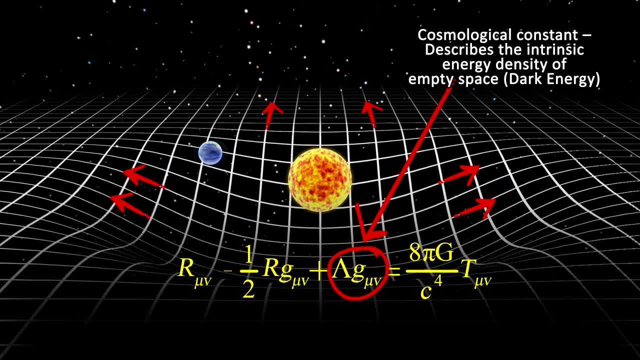 for what we observe as dark energy, the accelerating expansion of the universe. It would comprise energy in opposition to gravity. Lambda is a very small number, about 1.1 times 10, to the negative 52 inverse meters squared At small distances, this effect is largely negligible. 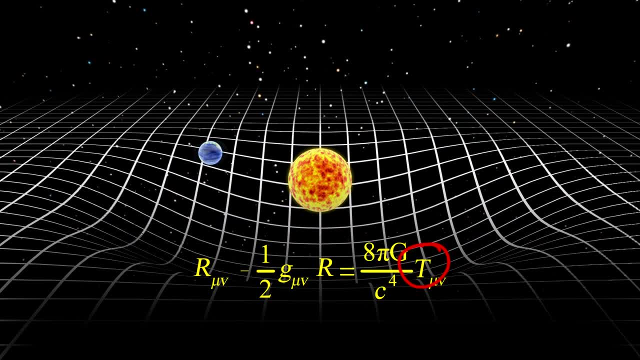 On the right side, t is the stress-energy momentum tensor, which tells us the density of energy and momentum at each point in space-time. It is the source of the curvature. There is also a constant which is equal to 8 pi g divided by the speed. 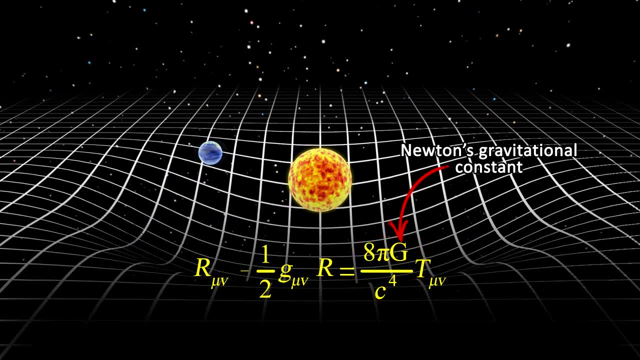 of light to the fourth power. g is Newton's gravitational constant, But this whole term is sometimes referred to as Einstein's gravitational constant. It's really just a conversion factor to make sure we get the proper units. The way these equations are formulated is: 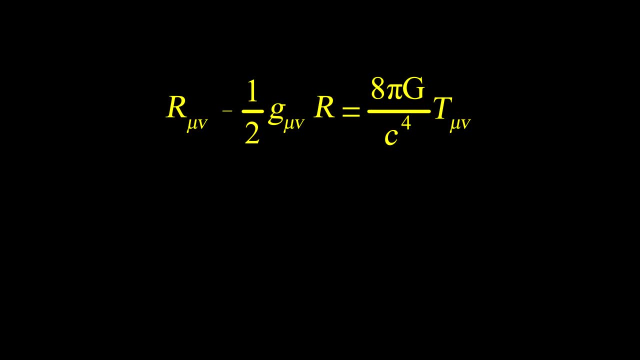 by treating the gravitational constant of the space-time curve. The equation is called the space-time in four dimensions: Three spatial dimensions and one dimension of time. This is incorporated in the mu and nu subscripts. The value of mu and nu can be zero, one, two or three. The 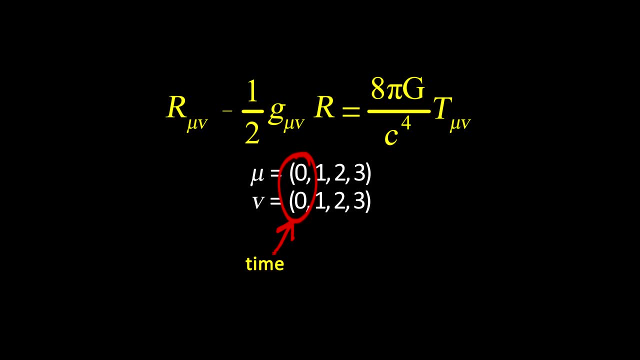 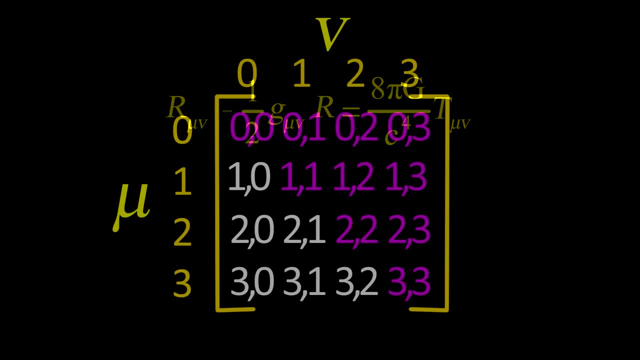 zero subscript conventionally represents time, and the one, two and three represent the three spatial dimensions. This is why we have ten equations. So, for example, if we draw a matrix of all the values that mu and nu could have, we would see that there are. 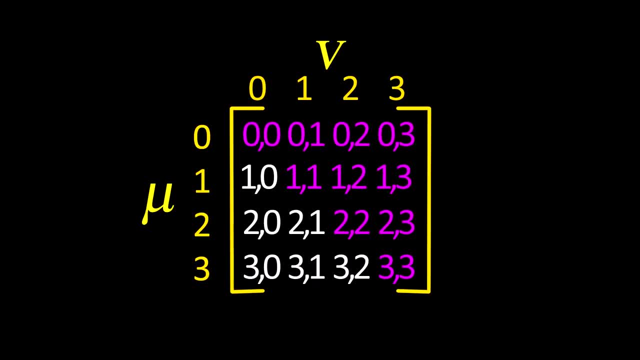 sixteen possible combinations. But this matrix is symmetrical, so zero and one, for example, is equivalent to one and zero. So if we take all the non-symmetrical combinations, we come up with ten combinations, Hence ten equations. Let's look at what some of these combinations mean. 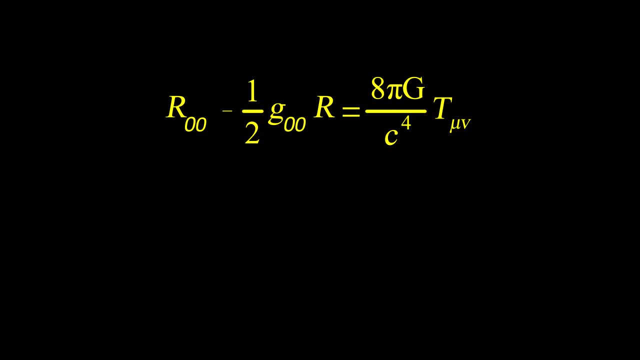 So, for example, one equation is where mu and nu are zero and zero. Zero represents the dimension of time. What this would describe on the left side is the speeding up or slowing down of time at a point in space, And the right side would describe: 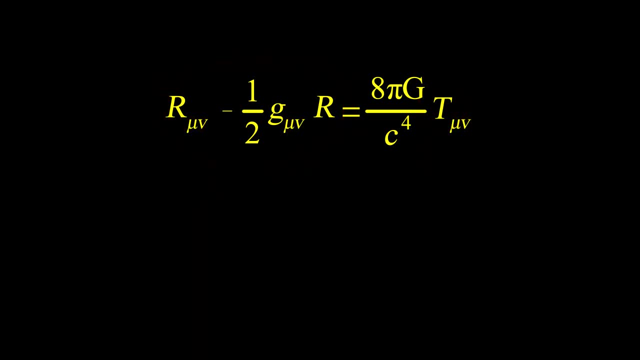 the energy at that point. Similarly, in another equation the value of mu and nu can be zero and one. This would represent time in one direction and one spatial direction in another. So the left side in this case represents the combination of the stretching of time with one spatial dimension. 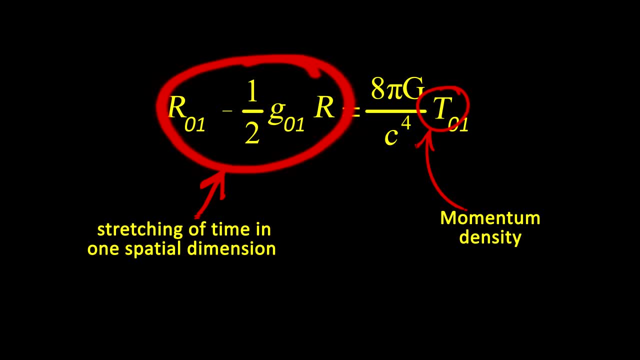 The right side in this case would be the momentum, or momentum density. In another equation, the value of mu and nu can be one and one. This would represent spatial dimension for both mu and nu. In this case, the left side is describing the stretching of space. 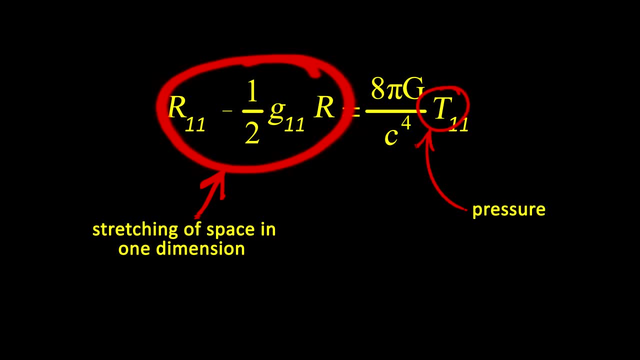 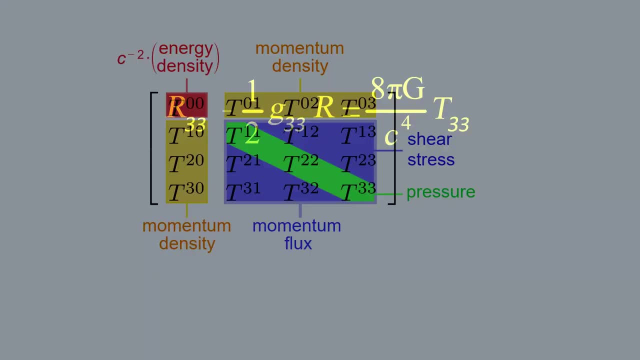 in one of the dimensions. The right side in this case, would describe the pressure at that point in space. The same can be said if mu and nu are two and two or three and three. Here's a matrix of what the various combinations of mu and nu mean for the stress-energy tensor. 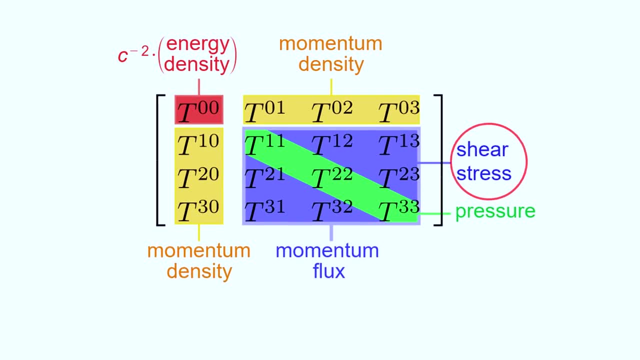 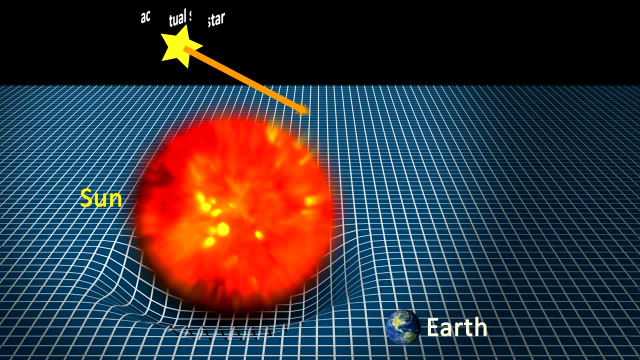 Note that the combination of the curvature and different spatial dimensions is called shear stress. Is general relativity true? Yes, in general. For example, it predicts the bending of light around massive objects- This has been observed for our Sun- as well as gravitational lensing around large clusters. 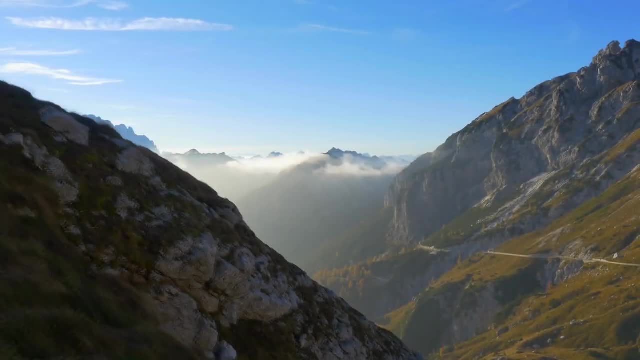 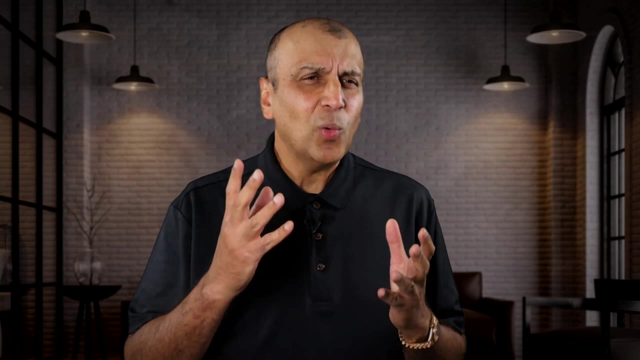 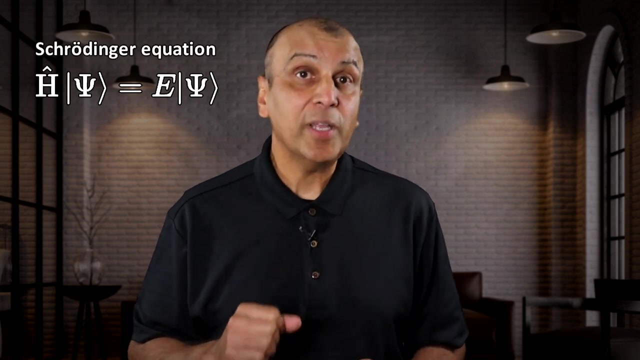 of galaxies. It predicts that time will run more slowly on the surface of Earth than on a mountaintop. This has been confirmed with atomic clocks, So why do we think that it's incorrect or at least incomplete? No one should take general relativity seriously. The problem is that it does not fit with what is. 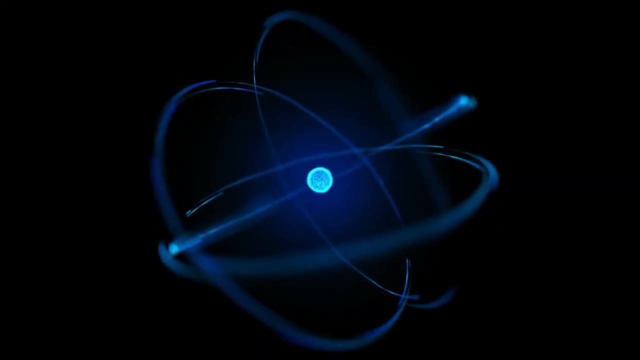 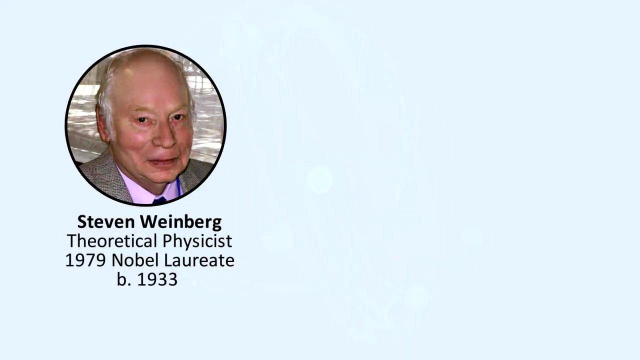 probably an even more accurate theory, and that is quantum mechanics. There is no theory that describes how gravity works at quantum scales or even very small scales. Nobel laureate Steven Weinberg, of electro-weak theory fame, said that no-one should take general relativity seriously. 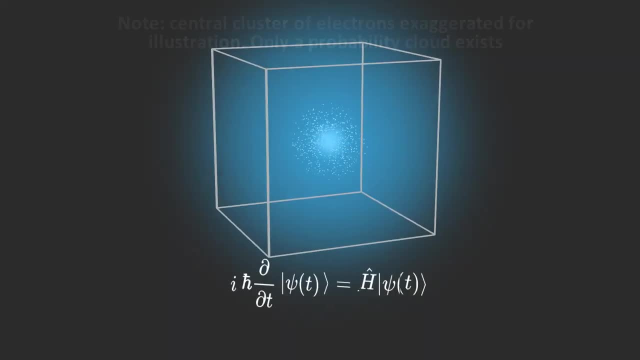 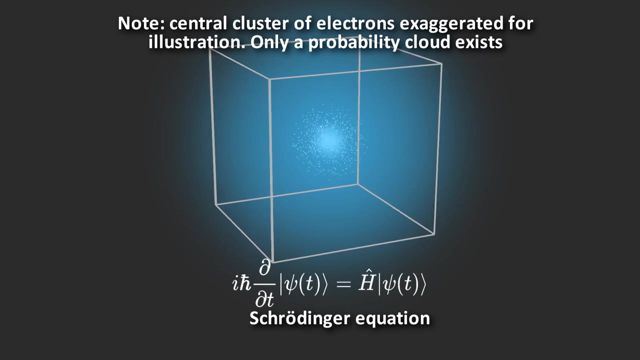 for distances shorter than about 10 to the negative 35 meters. So for example, let's take of one electron and one proton. Quantum theory says that the electron is in a superposed state, meaning it is in multiple positions at various distances from the nucleus at the same time. 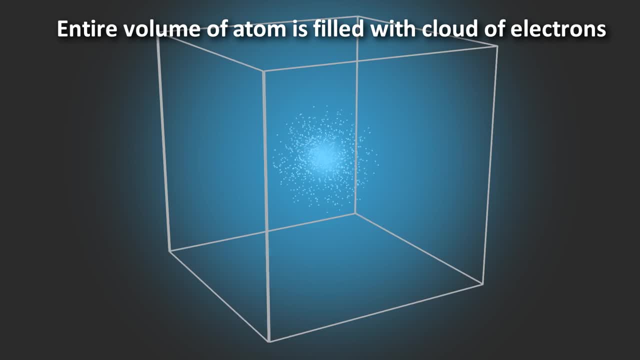 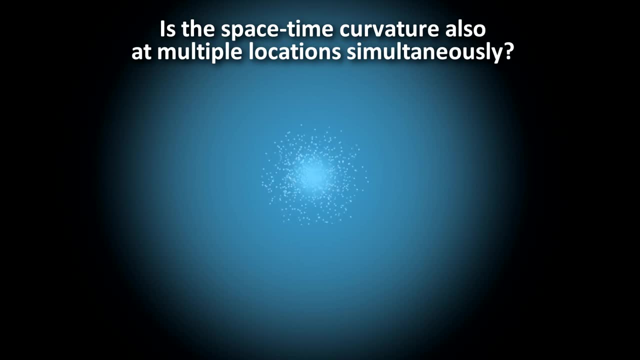 We only know the probability of finding it at a particular radius if we were to measure it. Since the electron has mass, according to general relativity it must curve spacetime, But it is in multiple locations at the same time. Then the question is: where is the curvature? 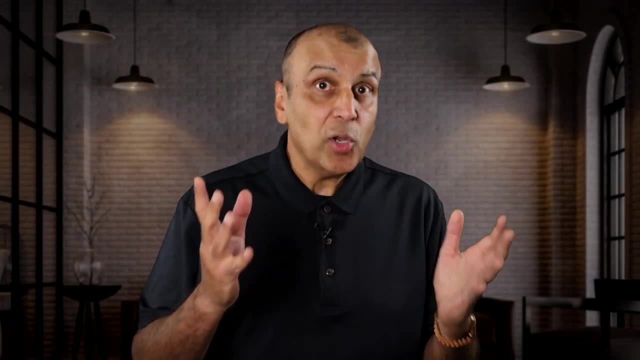 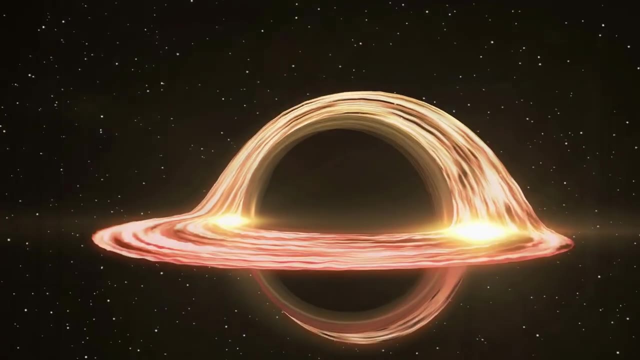 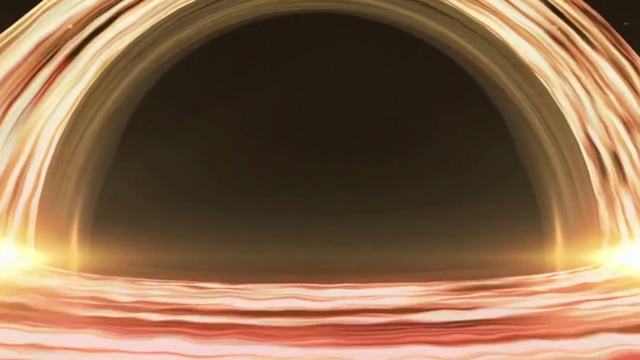 Is it also at multiple locations at the same time? We don't know. There's nothing in general relativity akin to superposition, like there is in quantum mechanics. A second problem occurs in the case of black holes. General relativity predicts matter and energy being compressed to. 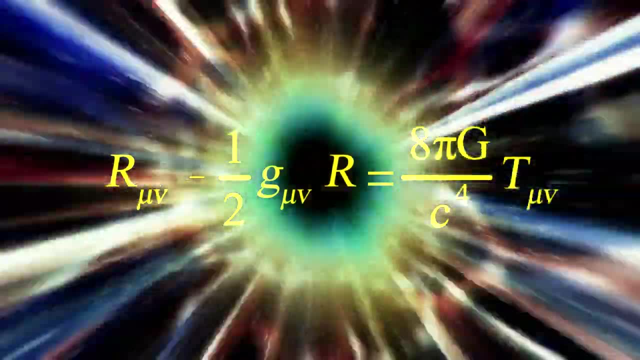 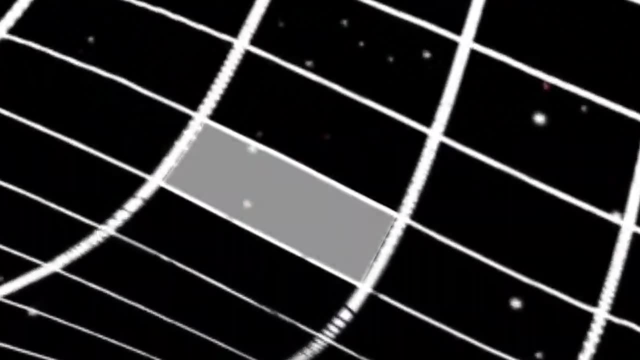 an infinitely small point in space with supposedly infinite curvature. But the theory breaks down the theory by saying that the electric field, that the electron moves in humans, belongs to a here. If you go back to our original equation of general relativity, it's easy. 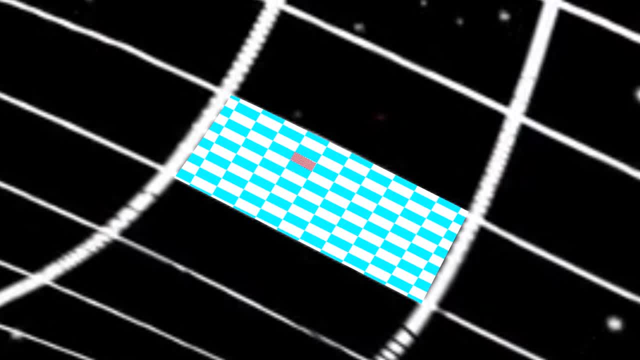 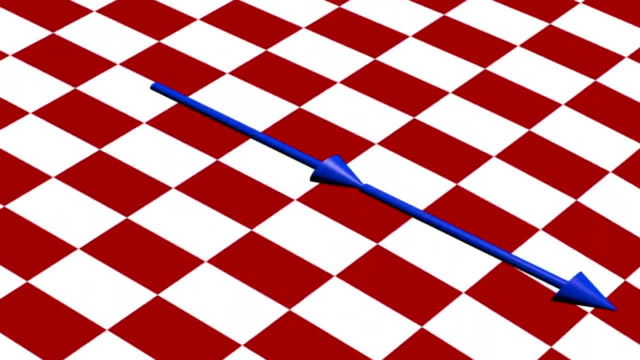 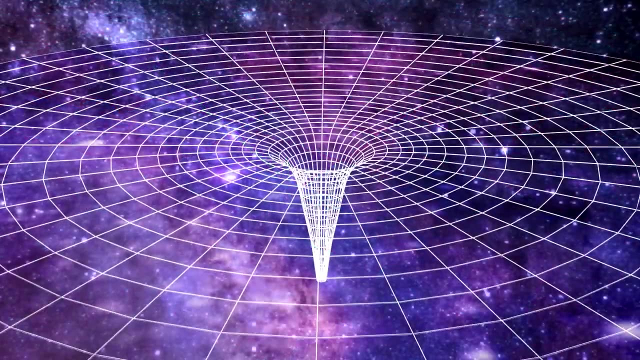 to see why it breaks down, since the equations treat spacetime mathematically as being flat at infinitesimally small distances and then calculate the overall curvature based on this presumption. A problem occurs when space is seemingly not flat at infinitesimally small distances. This 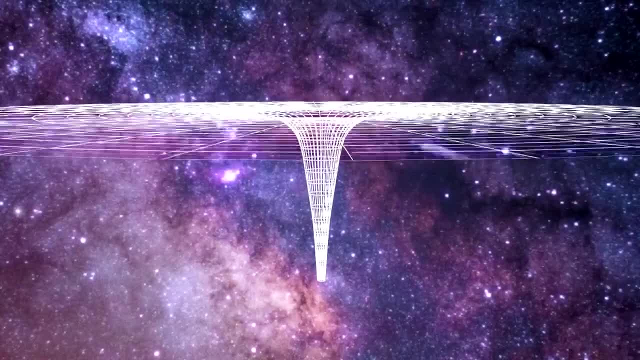 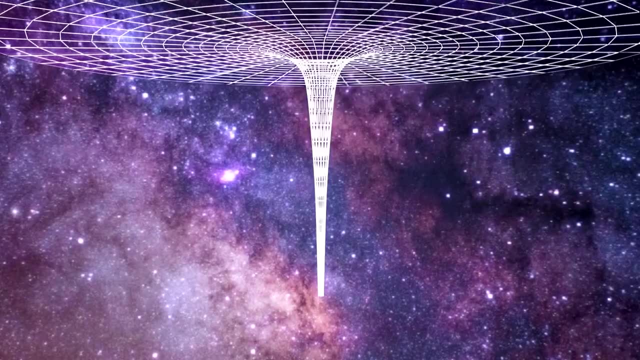 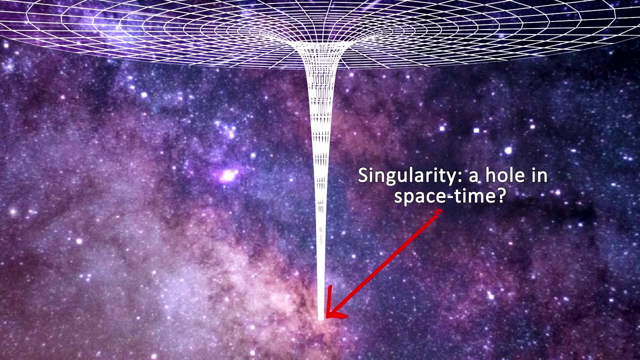 occurs at the singularity, since it's supposedly an infinitesimally small point. So how do you calculate spacetime curvature using flat spacetime with an infinitely curved point? It's a hole in spacetime. The mathematics of general relativity seem to describe singularities in this way, but